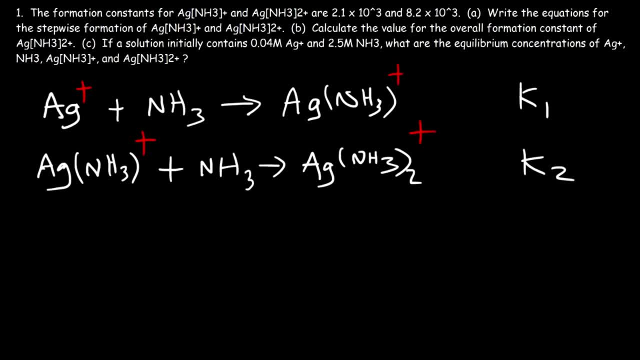 So that's how we can write the equations for the stepwise formation of these two complex ions. Now part B: Calculate the value for the overall, the overall formation constant of this ion. So what we need to do is add these two equations. 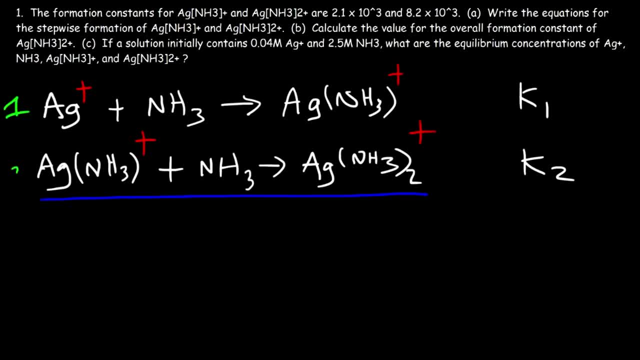 Let's call this equation one and two. Now, when adding these two equations, we can see that the intermediate will cancel, And so on the left side, we have the silver cation. By the way, everything is in the aqueous phase and these reactions are reversible, so we do need a double arrow. 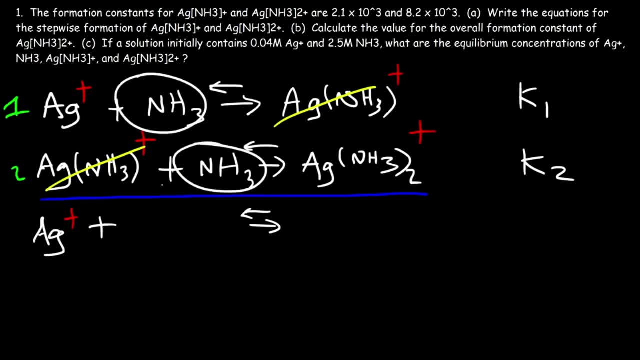 And then we have two ammonium molecules And this is going to give us the product AgNH3-2.. So let's call the equilibrium constant Kf for the overall reaction Now, because we added equations one and two to get the overall reaction. 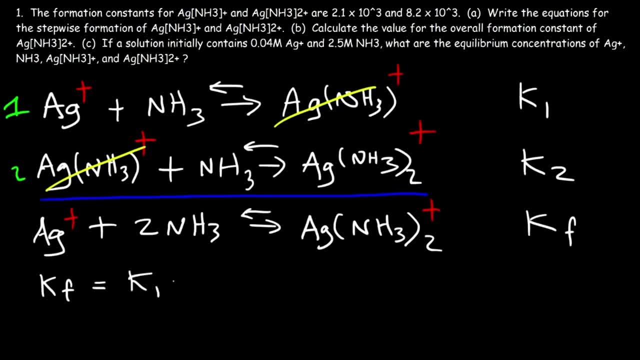 Kf is simply the product of the first two equilibrium constants, So it's going to be 2.1 times 10 to the third power, which is basically 2100, multiplied by 8.2 times 10 to the third power. 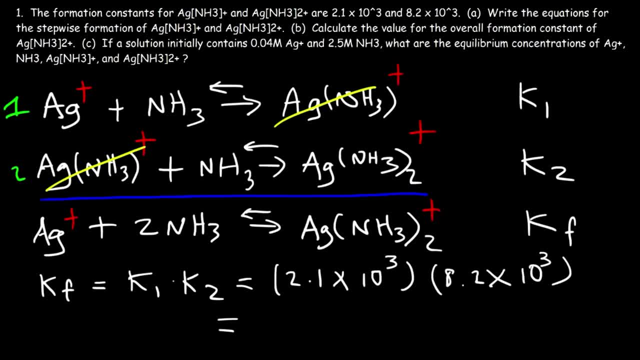 And that's 8200.. So 2100 multiplied by 8200 is equal to 1.722 times 10 to the 7.. So that's the value of the overall formation constant for the AgNH32 plus ion. Now let's move on to part C. 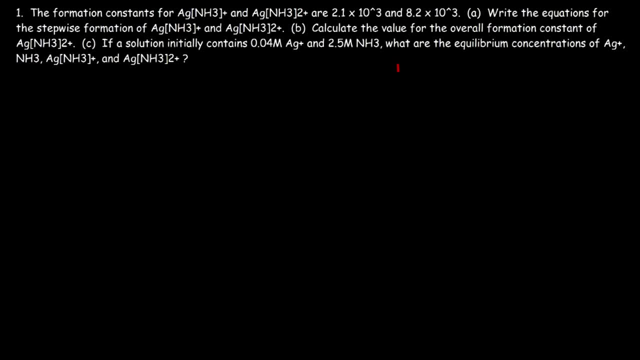 So I'm going to rewrite the overall reaction because we're going to need it at this point. So what we need to do at this point is we need to calculate the equilibrium concentrations of all species. We're given the initial concentration of the silver cation and the ammonia molecule. 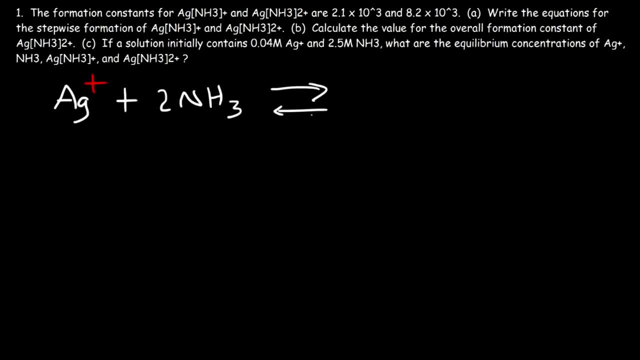 So what do you think we need to do in order to calculate the concentration of everything at equilibrium? Okay, So feel free to try it Now. because KF is so high in value, this reaction will essentially go to completion, And so, in this case, we need to use a BCA table. 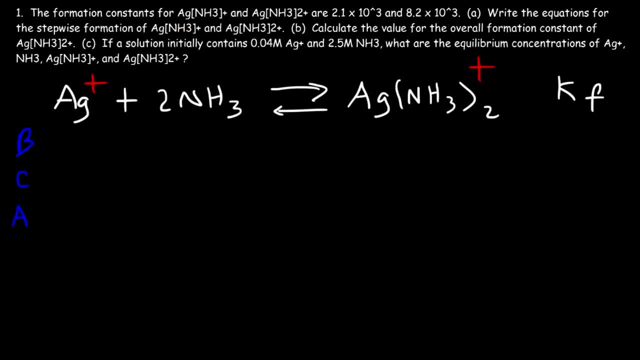 Now, if the volume is changing, you need to use the unit moles. If the volume is not changing, you could use moles or molarity. So in this example I'm going to use molarity. for this table Now, the initial concentration of silver is 0.04.. 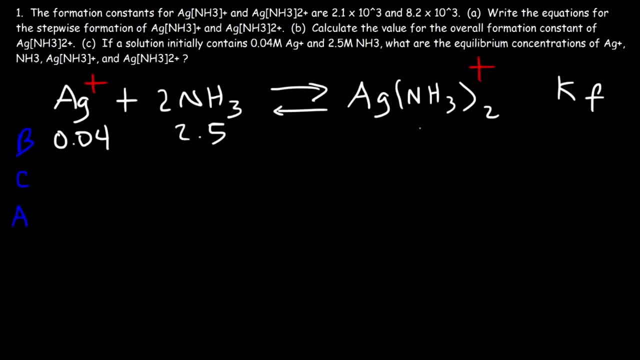 And for ammonia it's 2.5.. And this is going to be 0.. Now, because the reaction is going to go to completion, the amount of silver cation in a solution at equilibrium will be close to 0. So this is going to decrease by approximately 0.04.. 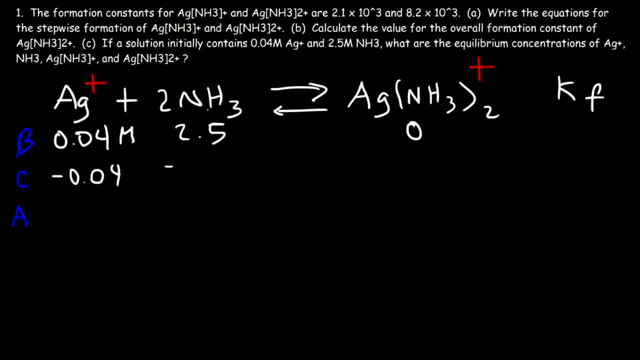 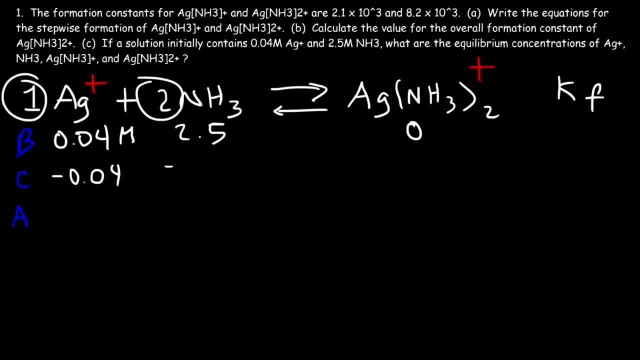 And notice the molar ratio: It's 1 to 2.. So if Ag decreases by 0.04, NH3 will decrease by 0.04 times 2, or 0.08.. And this will increase by 0.04, because it has the same molar ratio as the silver cation. 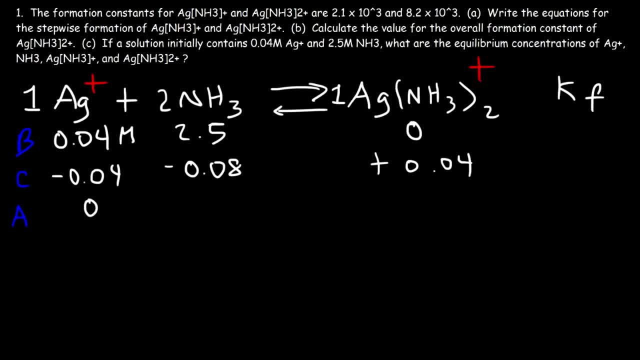 So this is going to go to virtually 0,, or a number close to 0. And then 2.5 minus 0.08.. 0.08., 0.08.. This is going to be 2.42, and this is just going to be 0.04.. 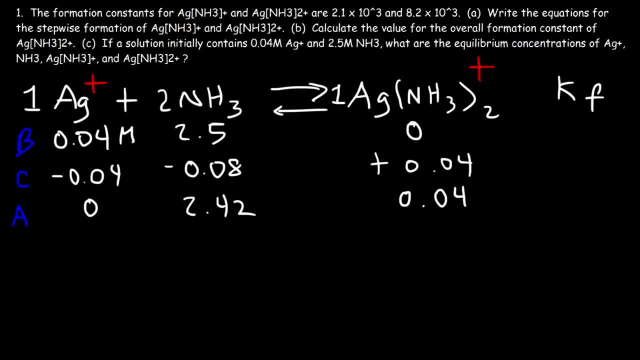 So at this point we already have the equilibrium concentrations of ammonia and of the AgNH3 2 cation. So the equilibrium concentration of NH3 is 2.42m And for AgNH3 2 cation, AgNH3 2 cation. 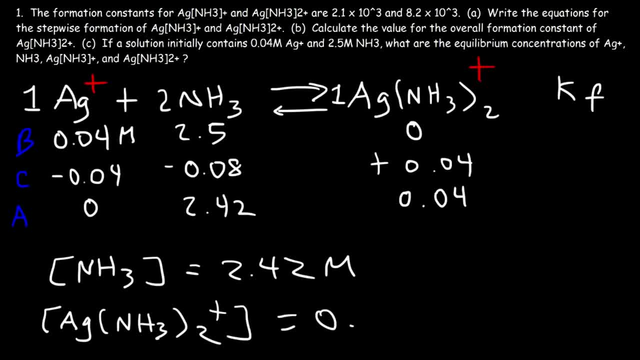 AgNH3 2 plus, It's 0.04.. So all we need to find at this point is the concentration of the silver cation and of AgNH3 plus. Now let's write the equilibrium expression for this reaction. So for any equilibrium constant, it's going to be the ratio of the products to the reactants. 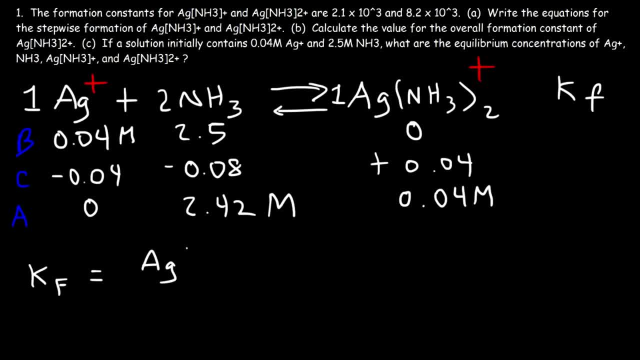 0.04.. So the only product that we have is AgNH3O2, and the coefficient is 1, so it's going to be raised to the first power. Now the reactants: we have Ag+ and also NH3. 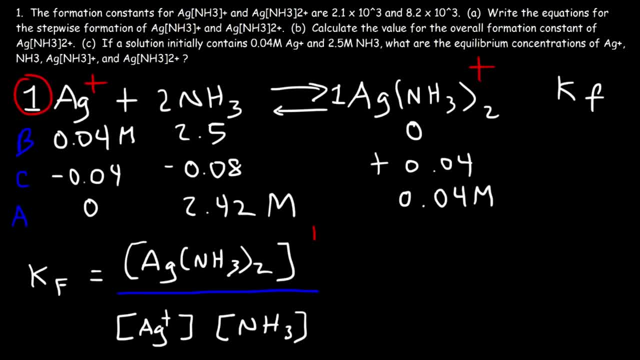 Now the coefficients are 1 and 2, so therefore, this is going to be raised to the first power and this is going to be raised to the second power. Now, KF, we know it's 1.722 times 10 to the 7th. 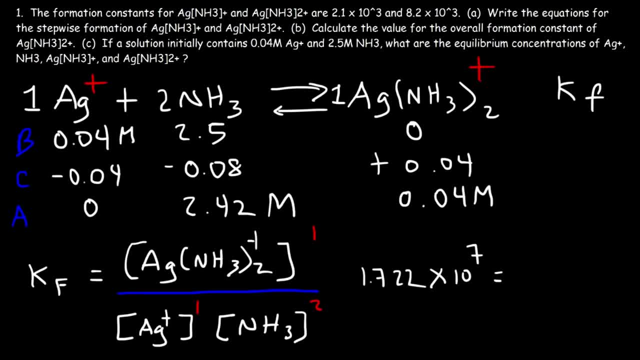 And the concentration of AgNH3O2, we have it as 0.04, so we can put that on top And on the bottom. we need to calculate Ag+ and we have the concentration of ammonia: it's 2.42.. 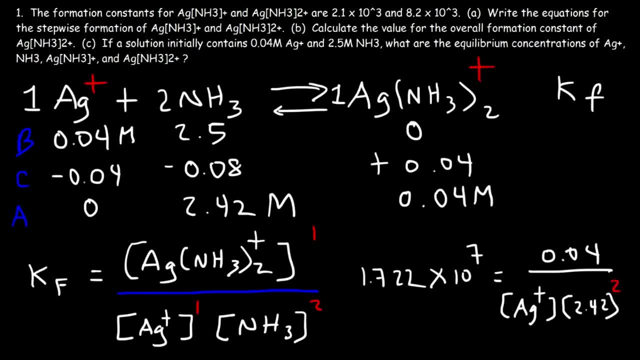 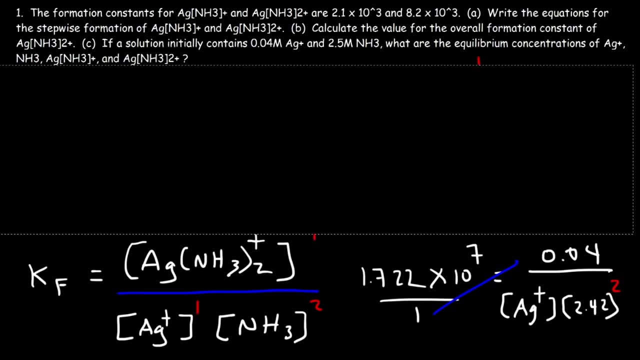 And let's not forget to square it. So at this point we just got to do math. So let's cross multiply. So 1 times 0.04 is 0.04.. And then we need to multiply 1.7.. 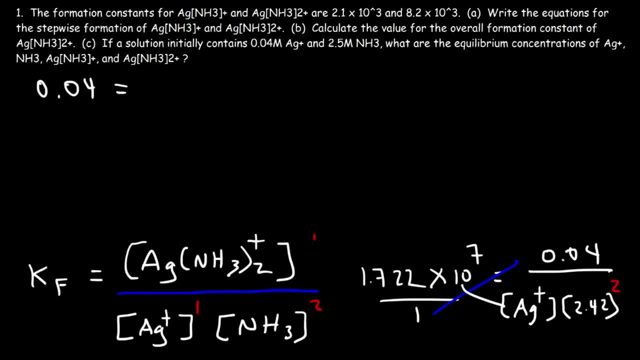 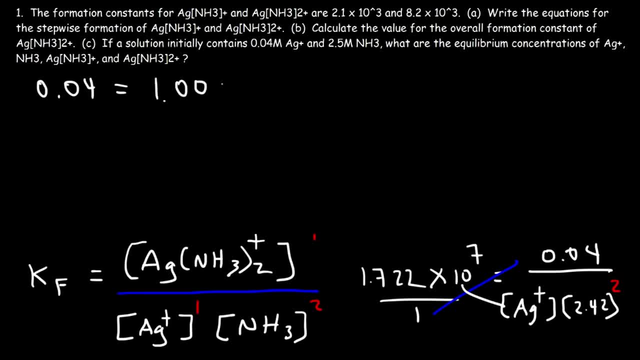 And so that's going to be 1.0085, if you round it times 10 to the 8.. Let's not forget, it's multiplied by Ag+. So to calculate the equilibrium concentration of Ag+, it's equal to 0.04 divided by 1.00.. 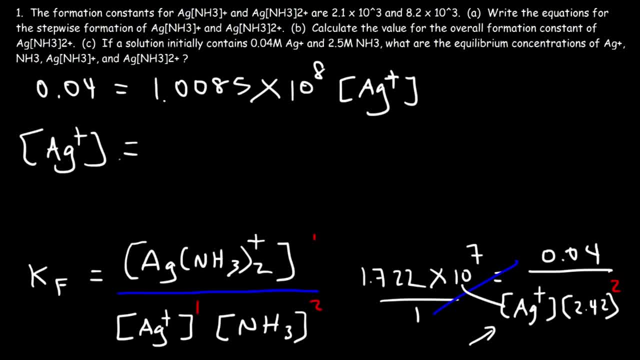 0.085 times 10 to the 8., And so the silver cation, the concentration at equilibrium, is 3.966 times 10 to the minus 10.. And so that's the third answer that we're looking for. 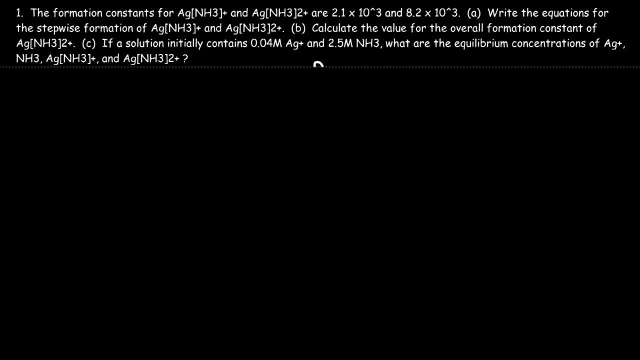 Now to calculate the last species, which is AgNH3.. We could use the first one, We could use the second one, We could use the third one, We could use the third one, We could use the reaction associated with K1 or K2.. 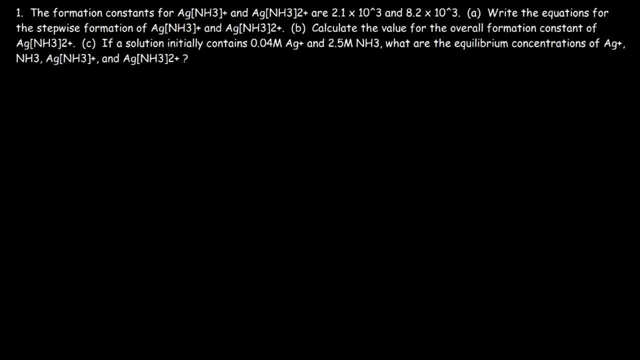 But to make sure our work is correct, we're going to use both equations And we need to make sure that the answer is the same both times. So let's start with the first stepwise formation of this species. So it was Ag+ reacting with NH3. 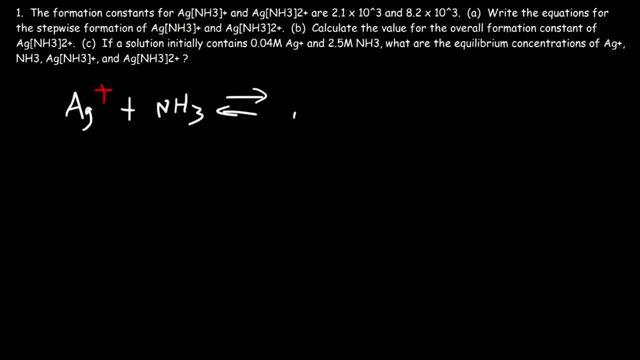 And that turned into Ag, And so this was associated with K1.. So K1 is going to be AgNH3+ divided by the concentration of Ag+, multiplied by the concentration of ammonia, So K1 is 2,100.. 2,100. 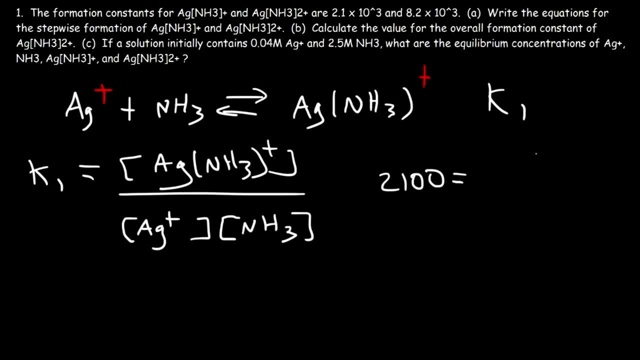 Our goal is to calculate this concentration, So I'm going to call it X, Or you can use another letter, if you want, Instead of writing this whole thing. Now we have the concentration of Ag+. Based on the last example, it was 3.966 times 10 to the negative 10.. 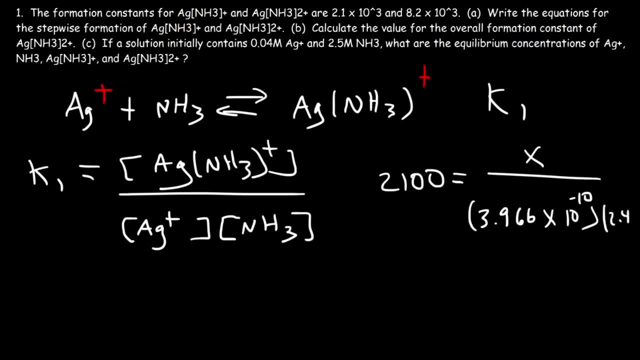 And then the concentration of ammonia is 2.42.. So let's cross, multiply: It's going to be 1 times X, which is X, And then we need to multiply those three numbers, So 2,100 times 3.966 times 10, to the negative, 10 times 2.42.. 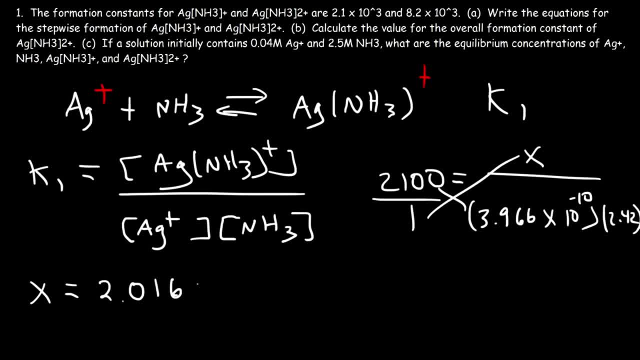 And so that's going to be 2.016.. Or we could just round that and say it's 2.02 times 10 to the minus 6 moles per liter. So that's the concentration of the first concentration, Complex ion. 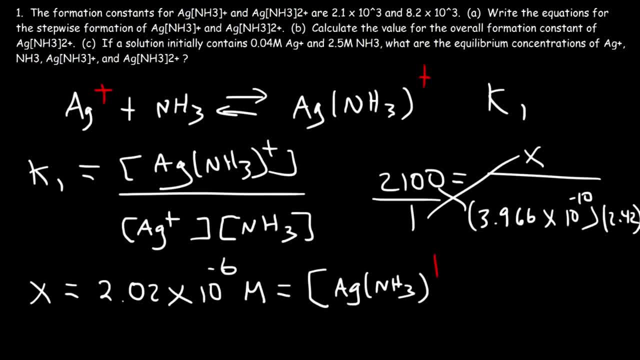 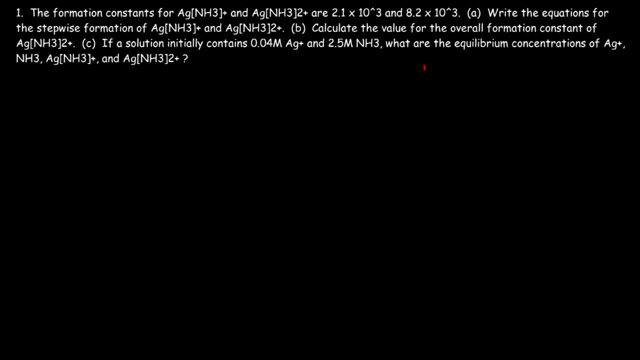 Ag and H3+. Now let's see if we can get the same answer using K2 as opposed to K1. If we get the same answer, then we know that the work is correct. So let's begin by writing the equation first. 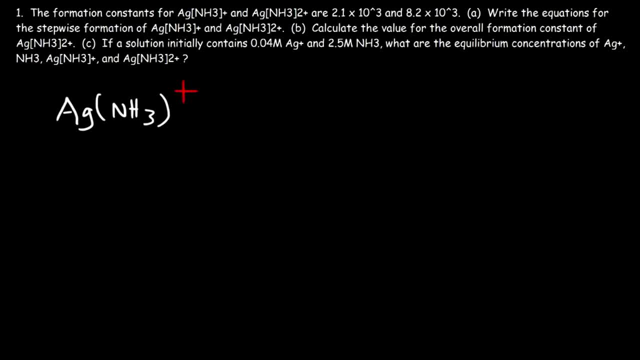 So we've got to start with this intermediate And then we're going to react So with another ammonia molecule, And so this time we're dealing with K2 as opposed to K1. And so K2 is going to be equal to Ag, NH3 2 plus divided by the first complex ion. 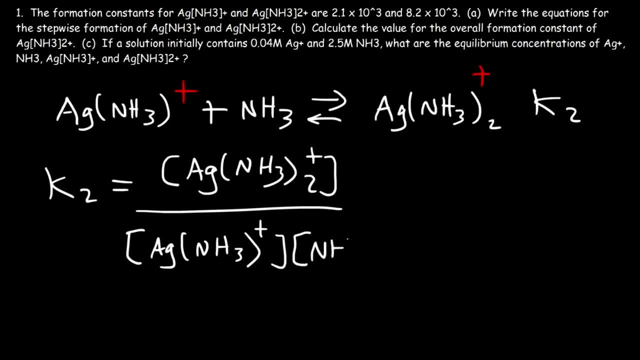 Multiplied by the concentration of ammonia, So K2, that's equal to 8,200.. And the concentration of this product? we know it's 0.04.. And our goal is to calculate this value, So let's call it X. 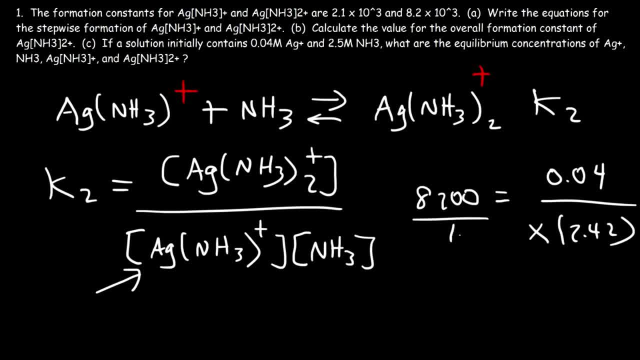 And NH3. we know it's 2.42.. So let's cross multiply So 1 times 2.42. Times 0.04.. That's going to equal that number, And then we need to multiply 8,200 by 2.42.. 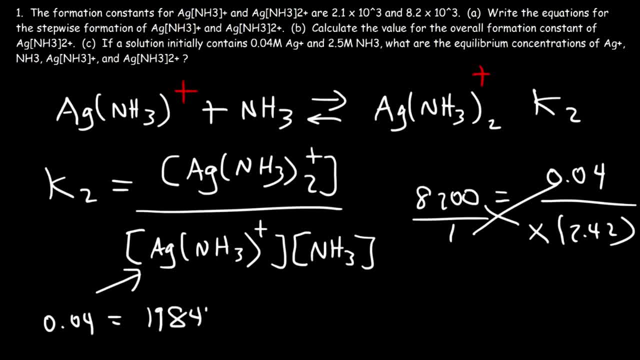 And so that's 19,844. Multiplied by X, So X is going to be 0.04 divided by 19,844.. And so you get the same answer: 2.02 times 10 to the minus 6.. 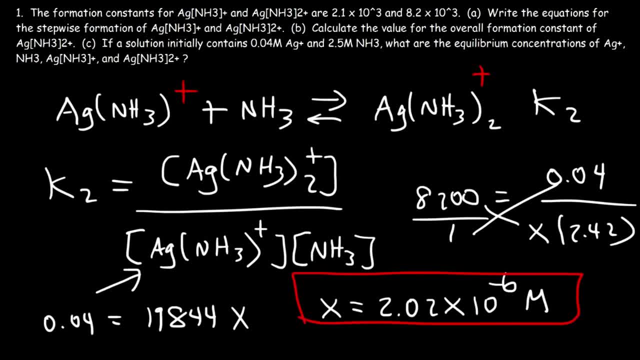 And so that's the equilibrium concentration Of the first complex ion, Ag NH3.. So now we have the values for every ion. So for NH3, we know it's 2.42.. For Ag NH3 2, we said it's 0.04.. 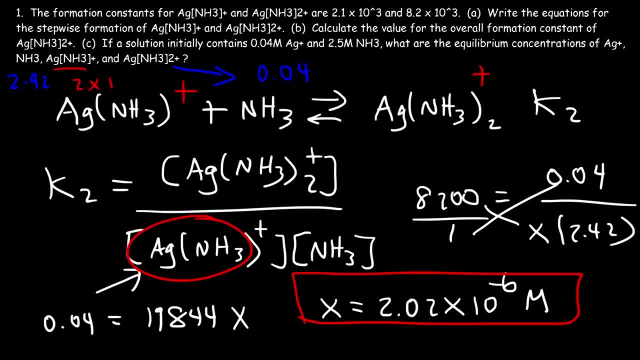 And for this one it's 2 times 10 to the minus 6. Which is basically close to 0. That's like 0.0000002.. And Ag plus is even smaller. That's very close to 0..